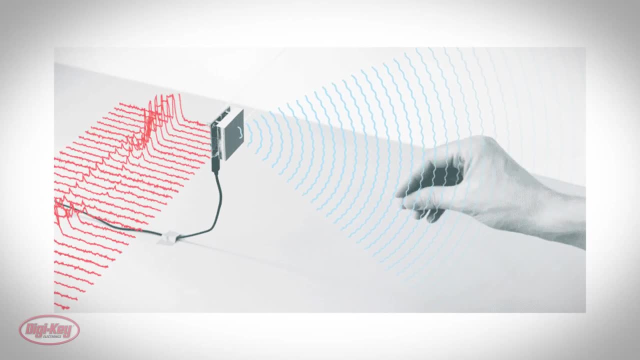 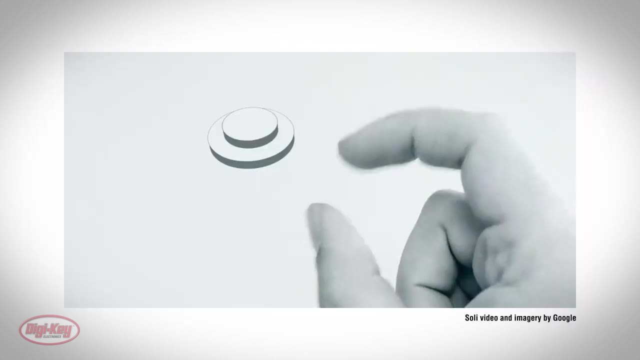 radar-based gesture recognition technology, which uses small high-speed sensors and data analysis techniques for detecting fine motions with sub-millimeter accuracy. As an example, Soli allows users to issue commands to a computer by rubbing a thumb and forefinger together in 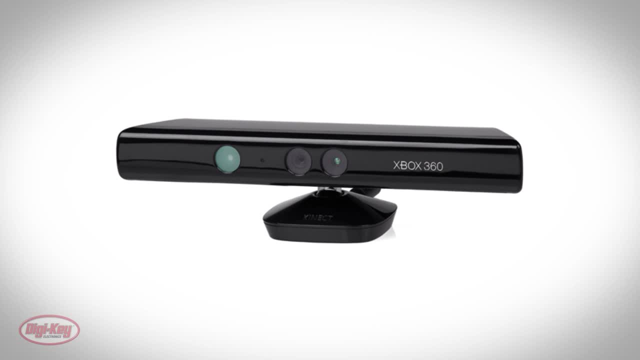 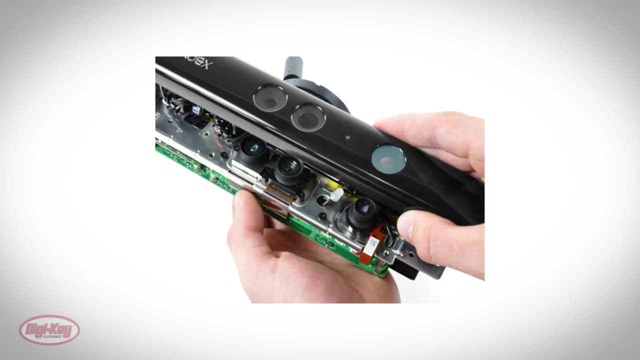 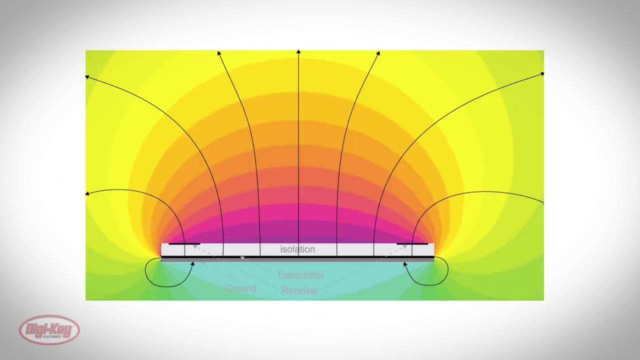 predefined patterns. Camera-based or vision-based gesture recognition technology uses a camera or cameras to capture and drive human movements. Both 2D and 3D cameras can be employed together with 3D vision for translating human gestures. Electrical near-fields or e-fields. 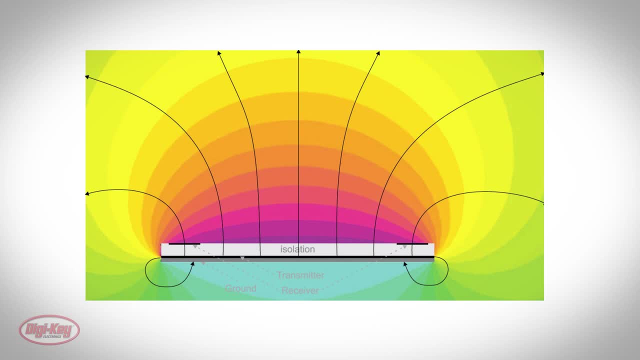 are generated by electrical charges and propagate three-dimensionally around the surface carrying the electrical charge. When an alternating voltage is applied, the resultant e-field is also alternating, And when the alternating wavelength is much larger than an electrode geometry, the result is a quasi-static electrical near-field that can be used for sensing conductive objects. 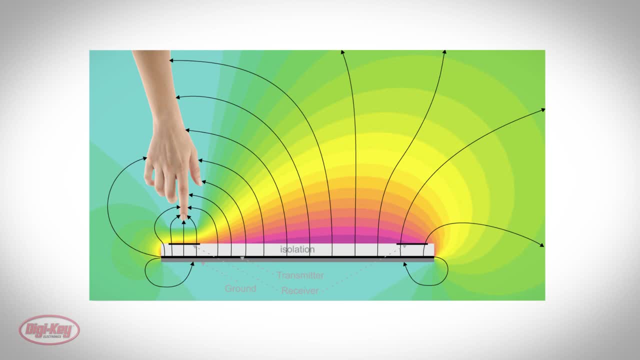 such as a human body. For example, when the operator's hand intrudes the e-field, the field becomes distorted. Specifically, the field lines interrupted by the hand are shunted to ground through the conductivity of the human body itself. As a result, the three-dimensional electric field 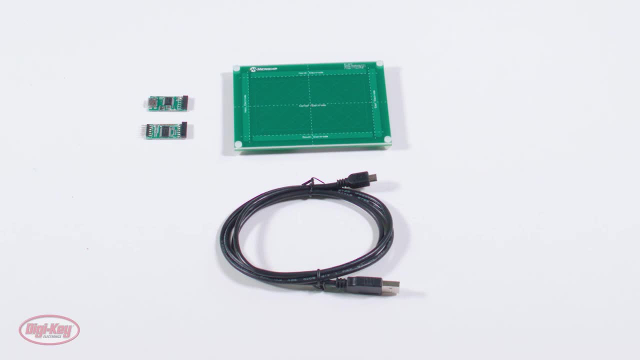 decreases locally And speaking of electrical near-fields. for gesture recognition, today's demonstration will focus on an evaluation kit that uses this type of technology. This is an evaluation kit using Microchip's MGC3030 3D Gesture Controller, which is based on their GEST-IC technology. 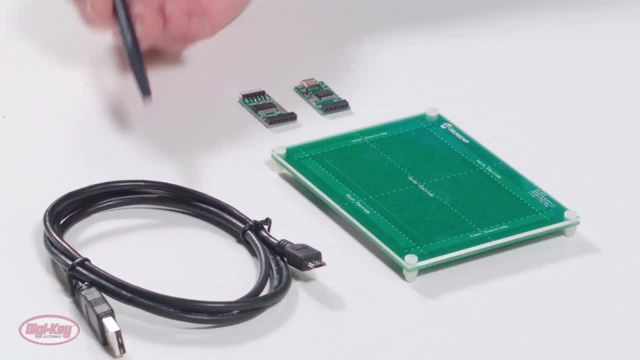 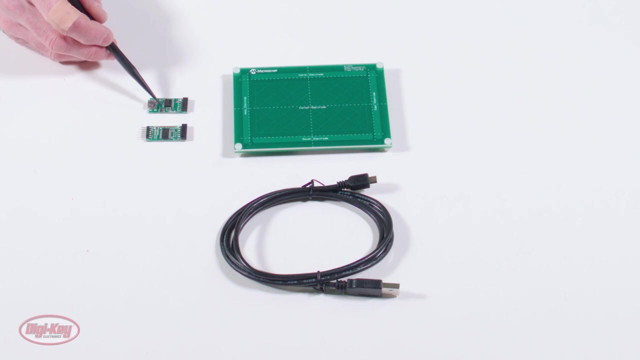 This evaluation kit will include a USB cable, an I2C to UART Bridge, the MGC3030 unit and the reference electrode PCB. The I2C to UART Bridge includes a PIC USB microcontroller, an LDO voltage regulator which converts 5V from the USB to 3.3V, a 6-pin socket for data. 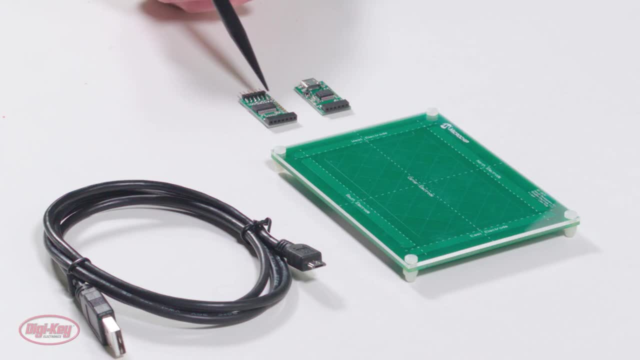 communication and power and a status LED. The MGC3030 unit includes the MGC3030 3D Gesture Controller, the PIC USB microcontroller, the 5V voltage regulator and the PCMC IC 3D1 controller. 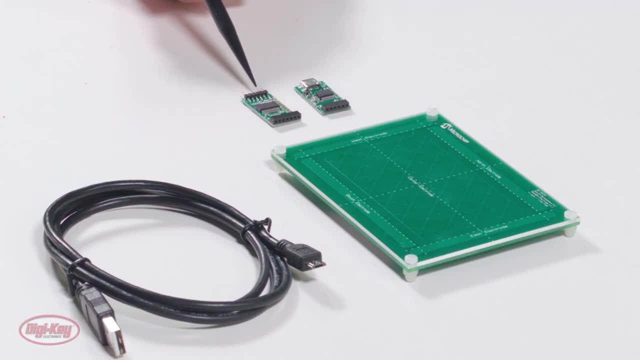 The MGC3030 unit includes the MGC3030 3D Gesture Controller, the PIC USB microcontroller, an LDO voltage regulator, 3D gesture controller, a 6-pin header for data communication and power, a 7-pin socket. 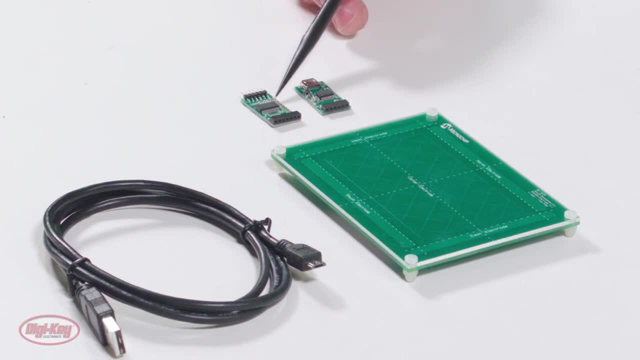 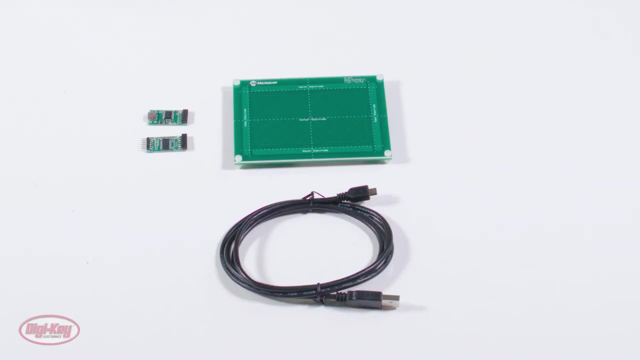 for interfacing with the electrode and it also has a status LED. The reference electrode PCB is a rather simple two-layer board design. The top layer includes five electrodes: north, south, west, east and center. The bottom layer is a ground plane with a single 7-pin connector. 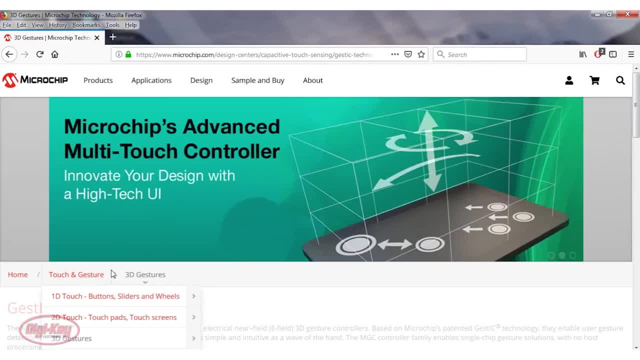 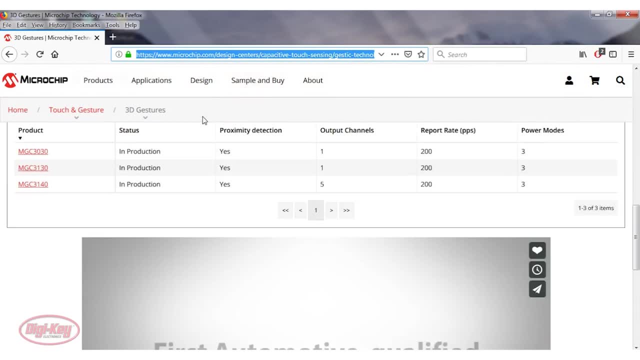 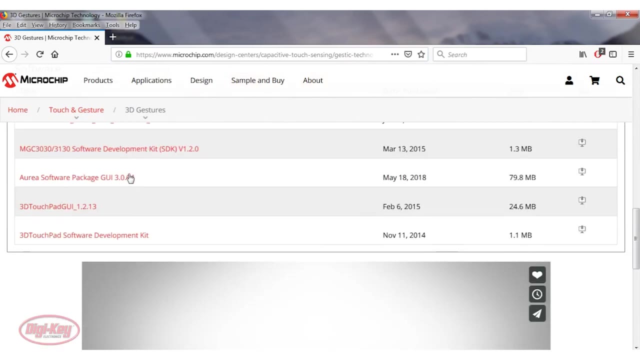 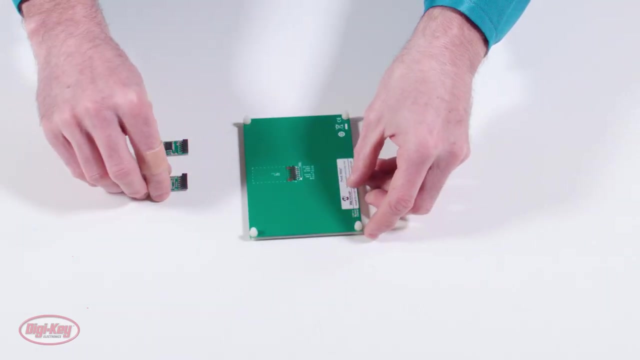 To use this evaluation kit, you must first download and install the ORIA evaluation software. Go to this website, scroll down to software. click on the ORIA software package GUI. download the file Before opening the software. connect the boards together and attach the USB cable. 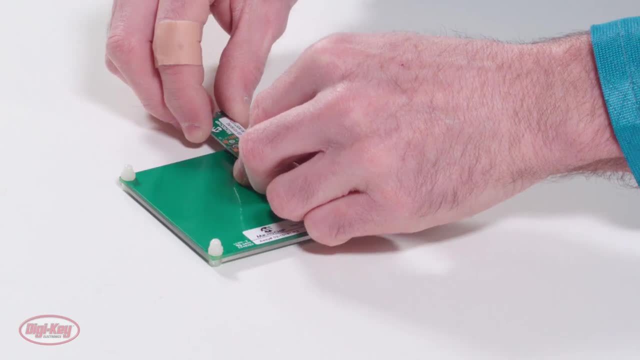 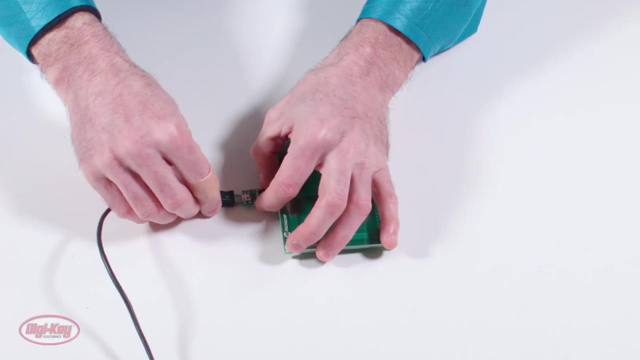 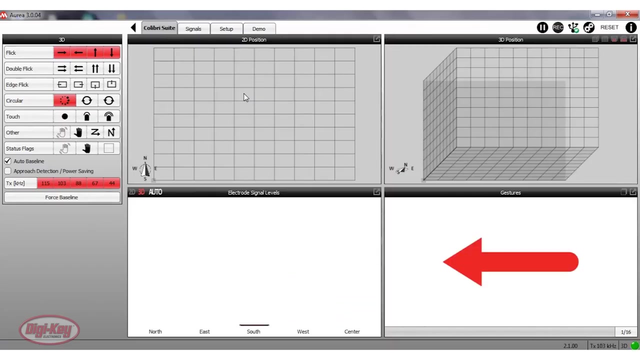 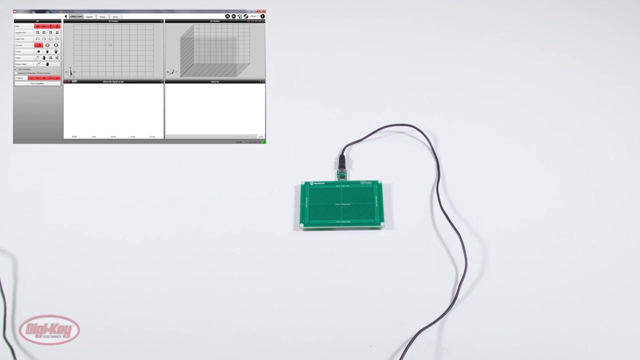 Okay, Let's see how it works With the software open. the Calibri Suite tab is open by default, which shows the output signals of digital signal processing. We can see how the signal level strength of the five electrodes change as I move my hand. 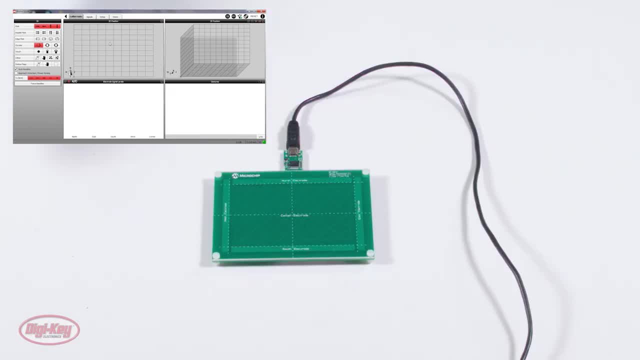 We can see various gestures In the gestures window. I'll swipe left, right, down and up. If I click on the two circular tabs, circular gestures will be detected. I'll make a counterclockwise gesture and a clockwise gesture. 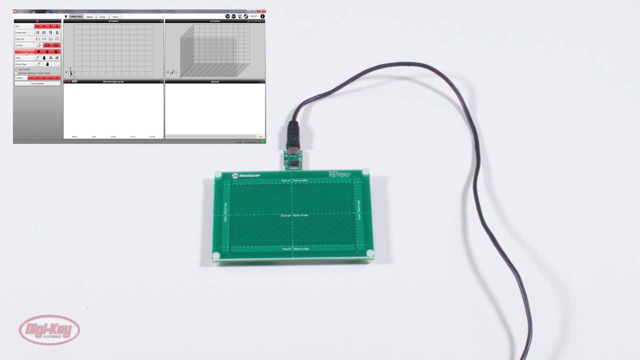 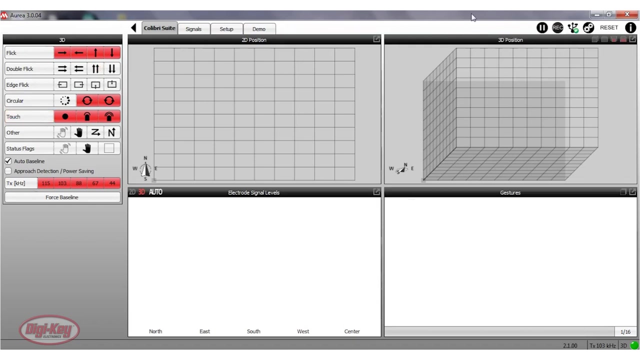 If I click on the touch tab, It will detect when I touch or tap the PCB. I'll tap the board once and I'll double touch. As you can see, there are additional gesture tabs And if you want to record logs, click on the record icon and name the log file. 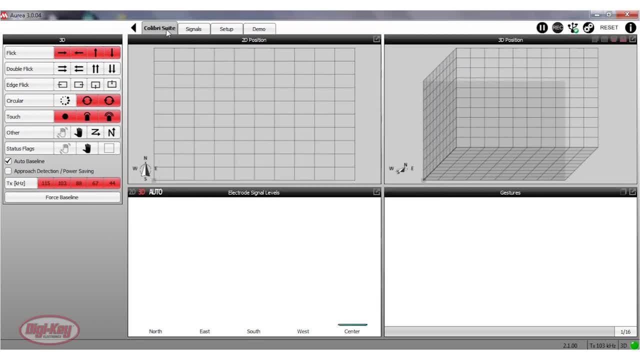 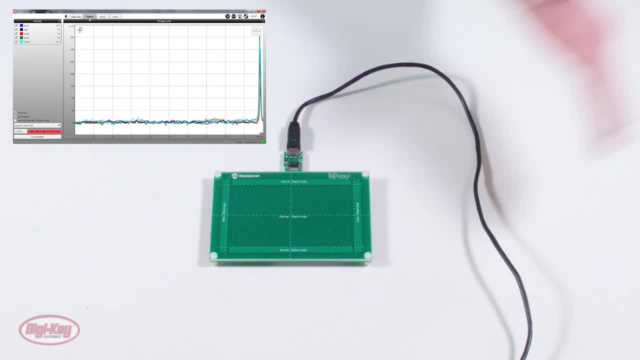 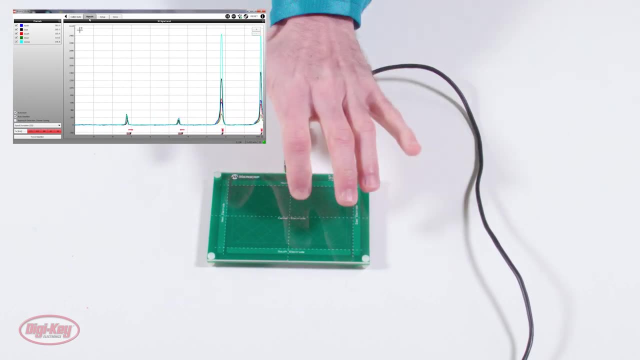 Finally, if we want to look at the plots of various sensor signals over time, click on the signals tab. The gestures are displayed on the bottom. I'll swipe left, right. I'll touch the board once and twice. I hope you enjoyed this video from Digi-Key. Thanks for watching.